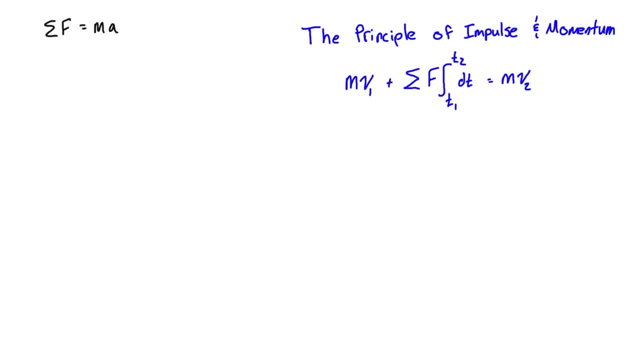 But if you've come to this video first, no problem, I'm going to go through it again. So we're going to write the left-hand side the same, and on the right-hand side we're going to rewrite acceleration as the change in velocity over time. dv dt. 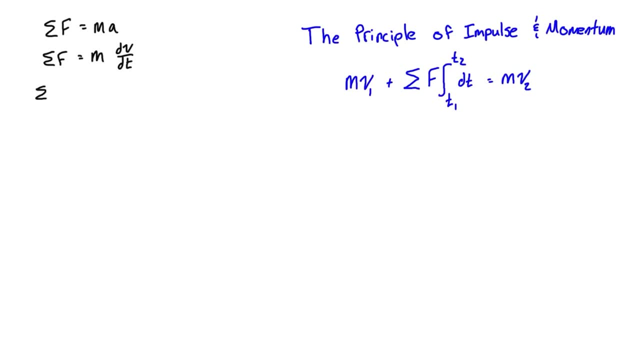 Then what we do is we multiply both sides by dt, So we have the sum of forces. dt is equal to mdv. All right, we want to integrate both sides, So we have our integral sine, and fdt is equal to integral sine of the right-hand side, mdv. 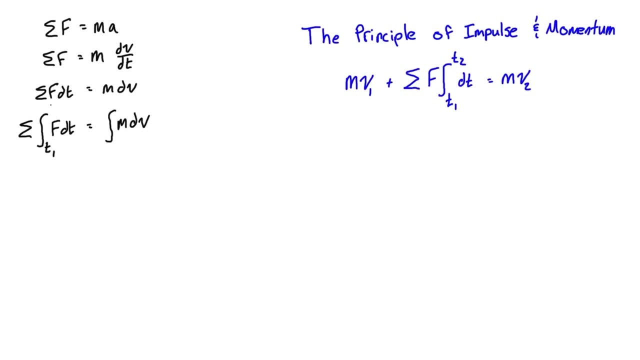 We want to take this as the definite integral, so we'll have from t1 to t2 and from v1 to v2.. It is important just to quickly mention that v1 is equal to velocity at t1 and v2 is equal to velocity at t2.. 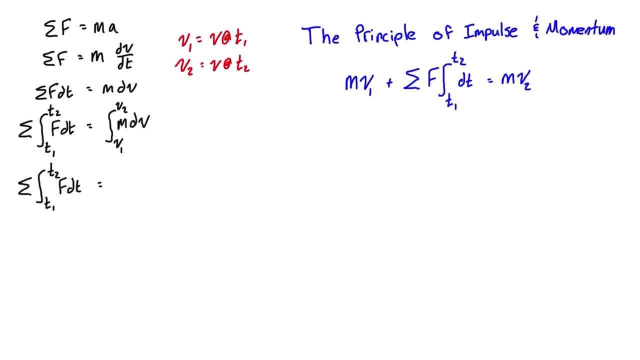 All right, so let's leave the left-hand side the same and if the mass is constant on the right-hand side, we can bring it out of that integral. This is going to be the case for a lot of impact and impulse problems and collisions. 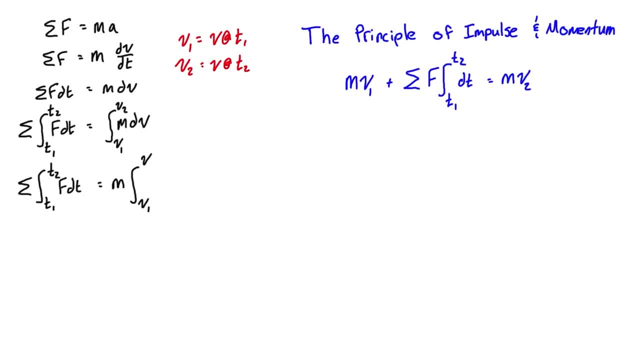 The only time really, and at this level, that you'll be seeing problems with a non-constant mass would be things like rockets, where the rocket is burning some of its fuel that's on board and the mass of the whole thing is changing. But for simple things like car crashes, baseballs hitting baseball bats, 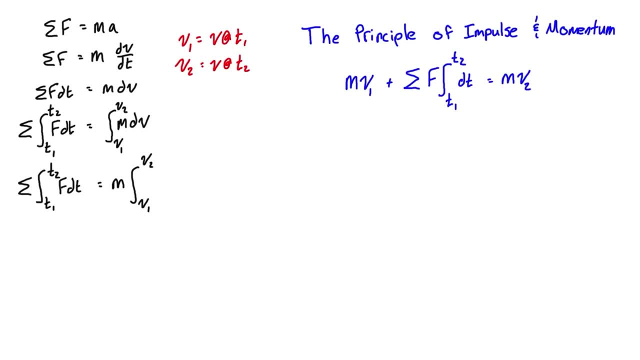 stuff like that. The mass will be constant, so we can just write that as the integral of dv. Again, we're not going to touch the left-hand side and we can really easily evaluate the integral of dv from v1 to v2.. 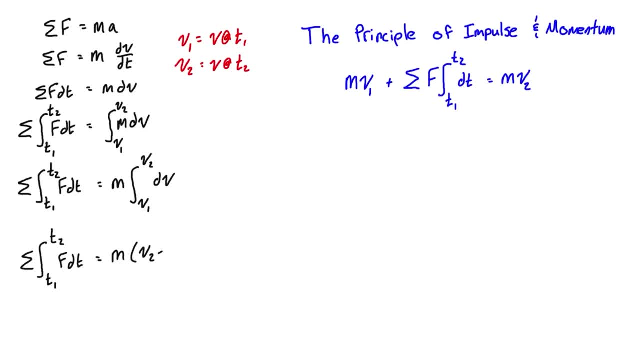 It's just going to be mass times, v2 minus v1, and we can just distribute the m through those brackets. So that's the right-hand side is also equal to mv2 minus mv1, and if we just bring the mv1 to the other side, 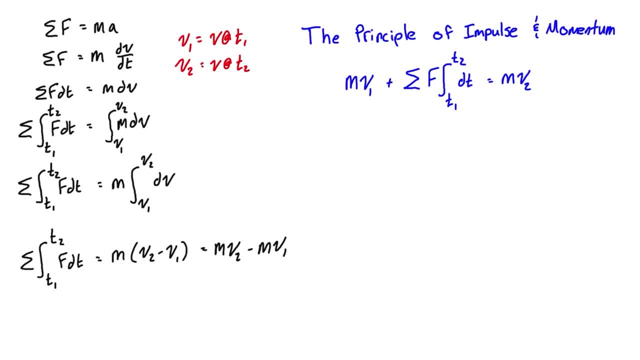 we get the principle of impulses and momentum as it's written in blue. So we have mv1 plus that integral is equal to mv2 and really what this is saying is mv1. this is the mass times, the velocity at time 1.. So mass times, velocity is.